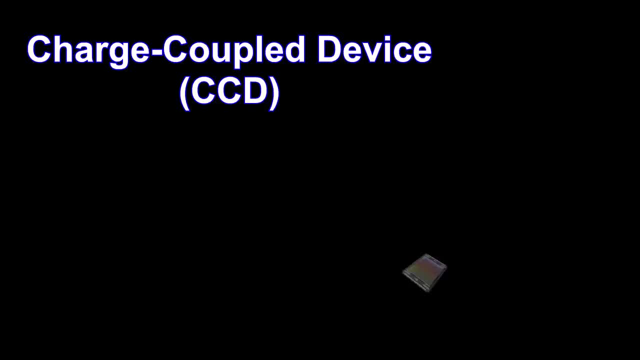 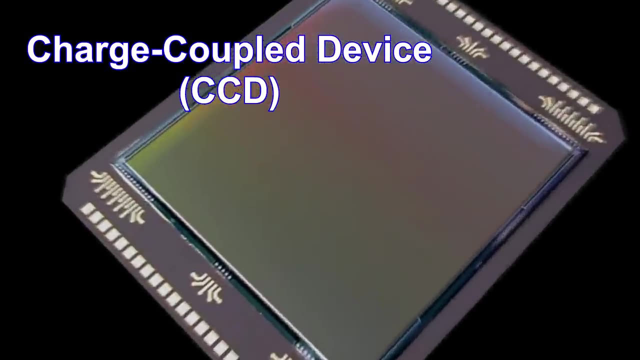 Of course, today's telescopes no longer use photographic plates. Instead, a charge-coupled device, or CCD for short, is used. These enable direct connections between an object's incoming photons and its image on a computer. Here's how they work. CCDs are based on a principle: 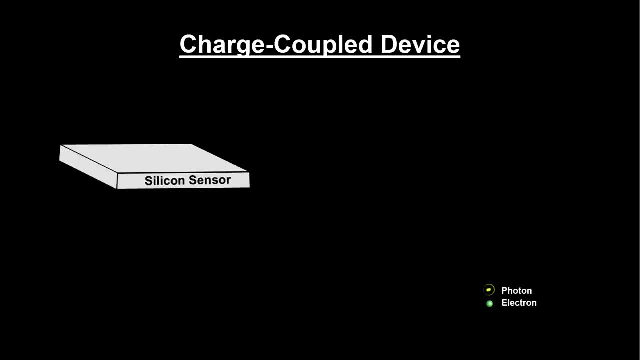 called the photoelectric effect. If a photon with sufficient energy hits an electron in the outer shell of an atom, the transfer of energy to the electron can be enough to free it from the atom altogether. This is a fundamental component of quantum mechanics, first analyzed by Albert Einstein in 1905.. CCDs use a thin wafer of silicon to produce 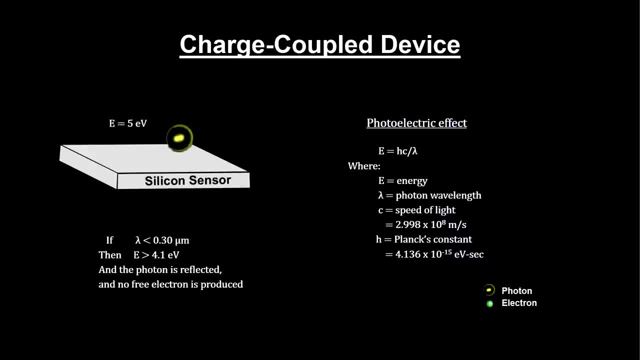 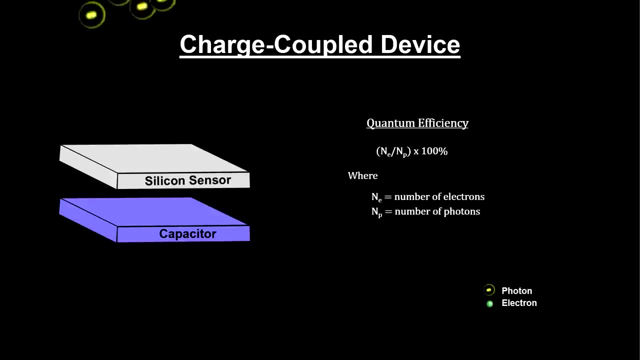 electrons from photons because silicon easily releases electrons with visible light. A tiny, positively charged capacitor can be used to produce electrons from photons. The capacitor is attached to the silicon wafer in order to collect the freed electrons. If we get one electron for each photon in the range, we'd have 100% quantum efficiency. 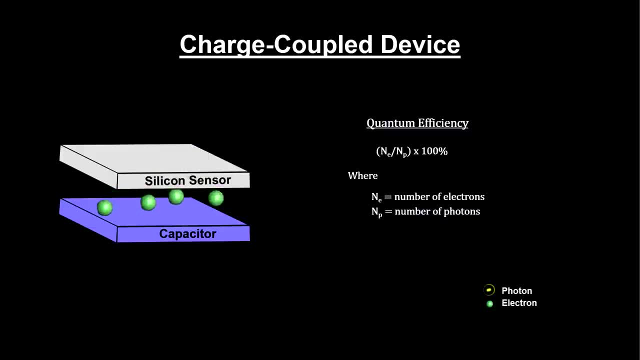 The highest quality CCDs can achieve up to 90% quantum efficiency. It's interesting to note that the quantum efficiency of the human eyes, rods and cones is only 1%. The photons start producing electrons in the outer shell of an atom and the electrons in the outer 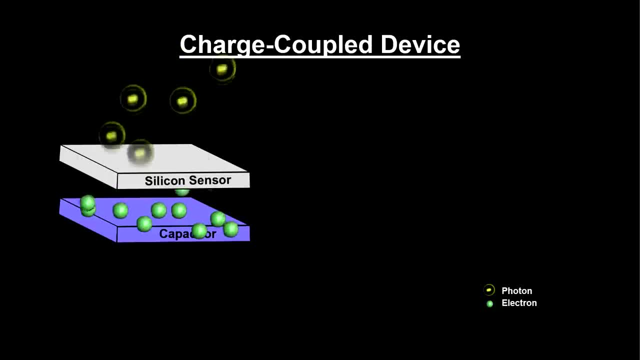 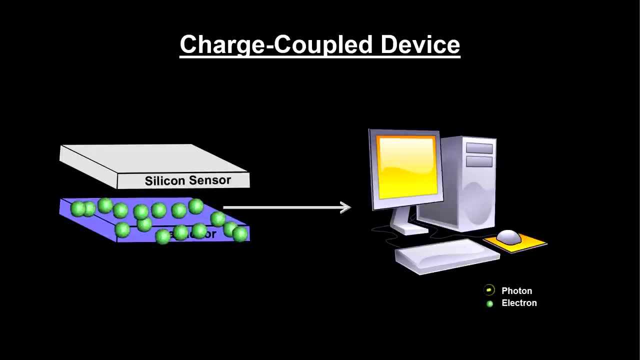 shell of the electron are the ones that create the electrons. As you start collecting electrons, the creator will start using his hands to carry them through electrons. The capacitor collects the freed electrons until the shutter is closed. At that point, the voltage across the capacitor represents the number of electrons the capacitor collected. 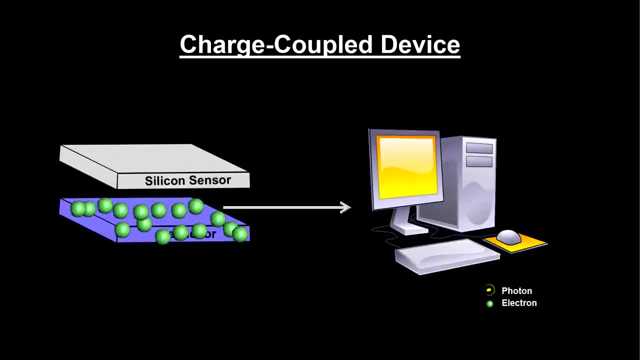 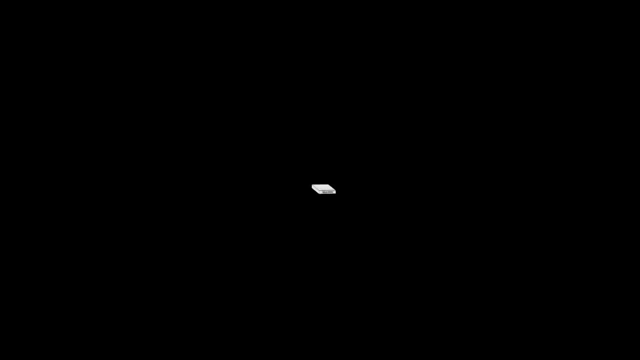 This information is sent to the computer. This information is miniaturized into an integrated circuit and represents 1 pixel. The first illusion of the electron is that there are neutrons in the circuit. CCDs are made of thousands or even millions of these, configured as an array.